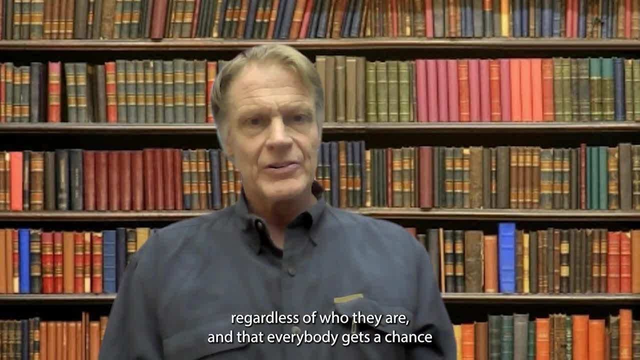 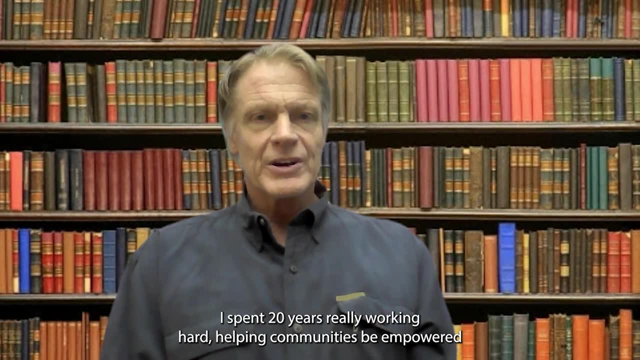 to have the same opportunities regardless of who they are, and that everybody gets a chance to thrive in their lives. I spent 20 years really working hard helping communities be empowered to do that, And then I came to Imagine and I saw something better, The kind 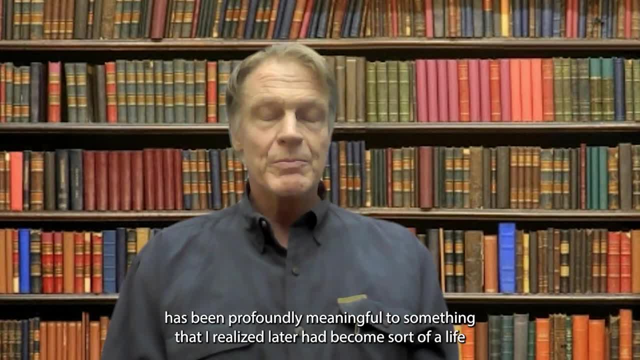 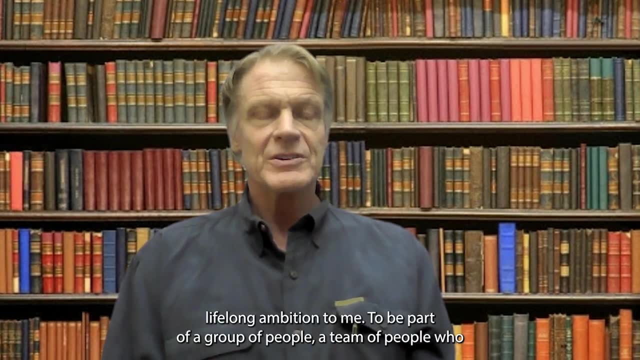 of work that Imagine does, and what Imagine has meant to me is it's been profound work. It's been really meaningful to something that I realized later has become sort of a life, life-long ambition to be, To be part of some, a group of people, a team of people who work. 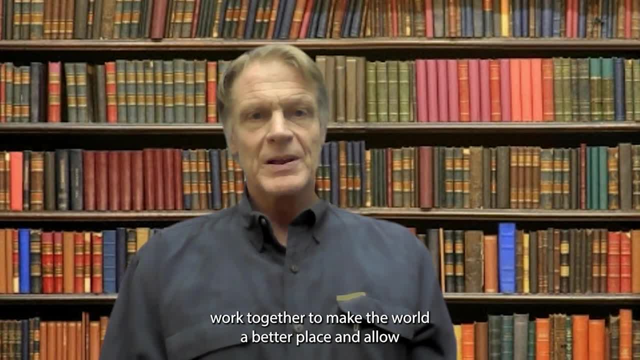 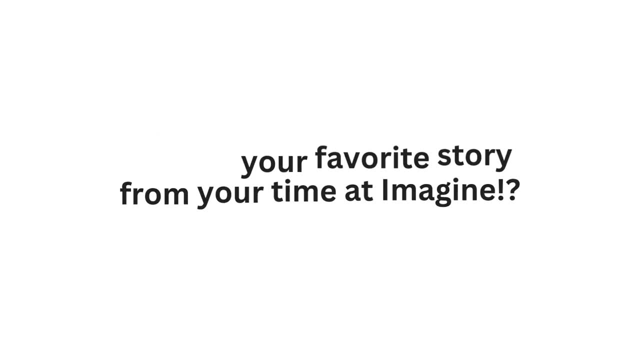 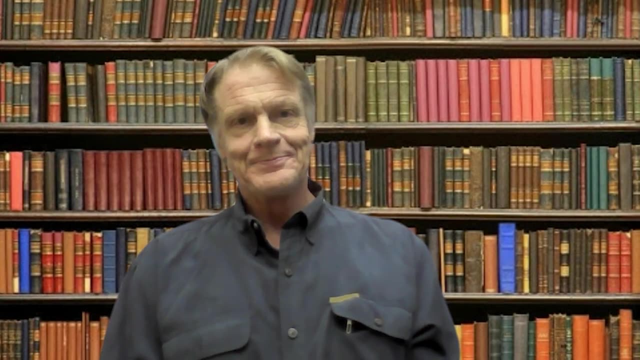 together to make the world a better place and allow the most marginalized amongst us to thrive. Jackie Free has brought on our foundation board, brought a connection to the community To imagine with Liberty Puzzles, who are the greatest puzzle makers, the greatest jigsaw puzzle makers. if you don't know them, you need to get to know them. they're amazing. 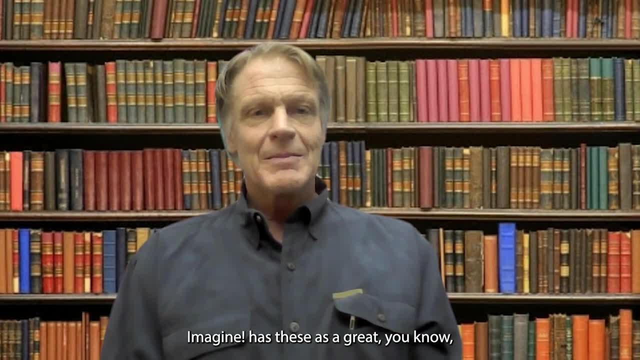 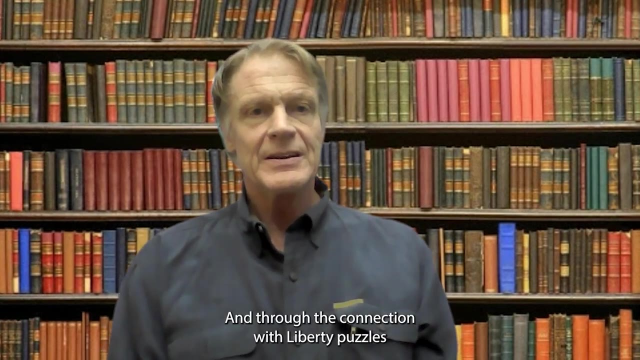 And you know, Imagine has these, has a great, you know, and part of people thriving is providing them with things they love to do. There are some amazing artists. Lana is one of them And, through the connection with Liberty Puzzles- the world's greatest puzzles- there is now a puzzle that is an Imagine puzzle that was painted by Lana. 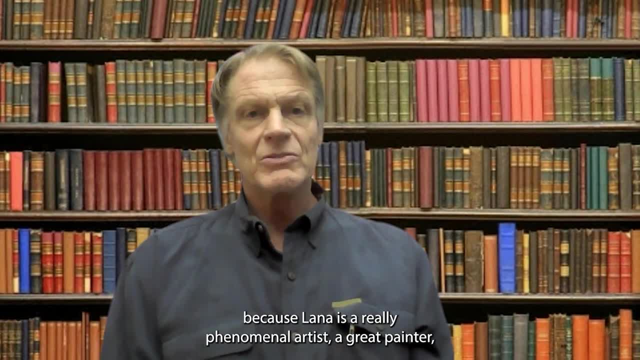 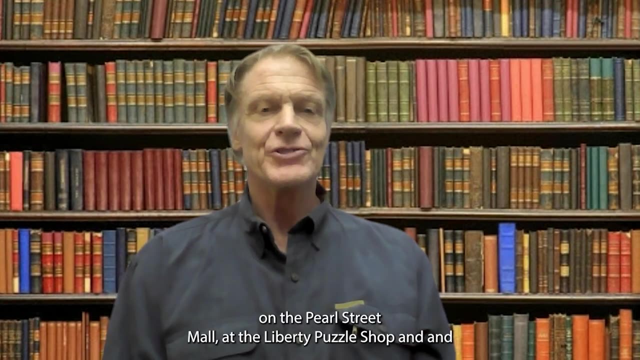 Because Lana is a really phenomenal artist, a great painter, really truly a great painter. She painted a beautiful painting that became part of this puzzle. I went down the morning. they were sort of celebrating that puzzle on the Pearl Street Mall at the Liberty Puzzle Show. 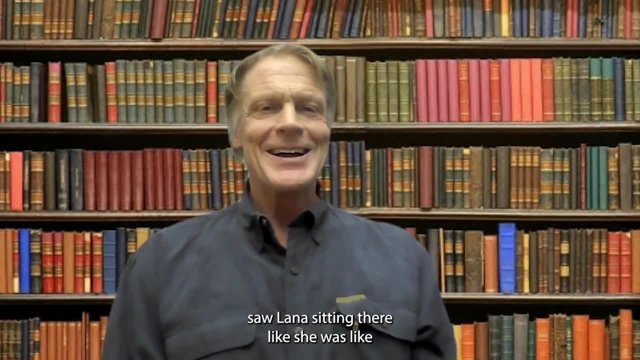 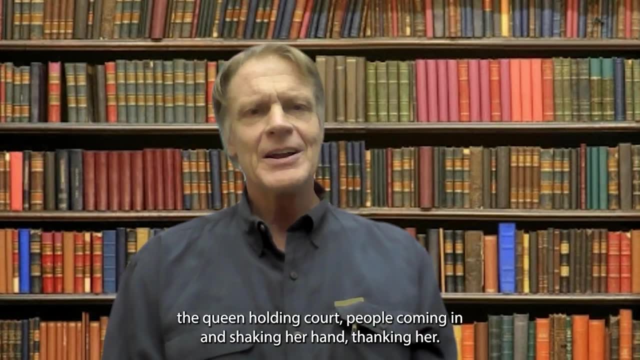 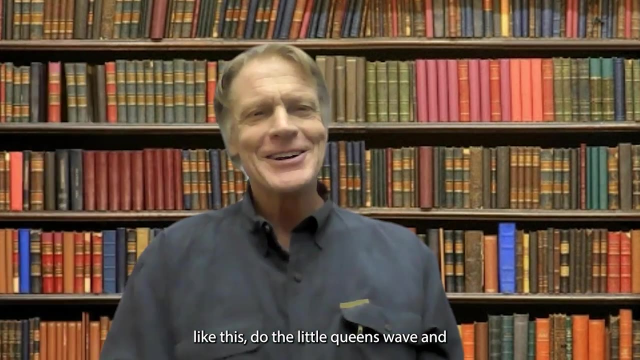 And I saw Lana sitting there Like she was like the queen holding court, People coming in and shaking her hand and thanking her And you know she would sort of nod and almost go like this: do the little queen's wave.